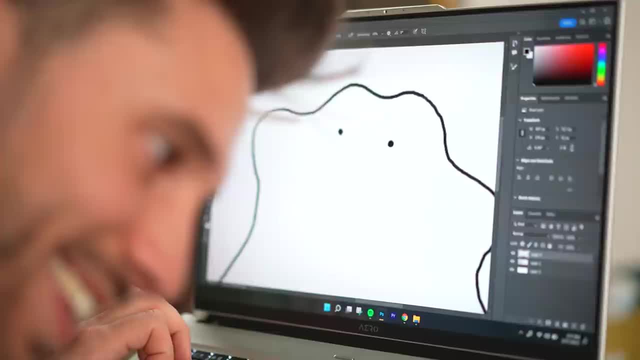 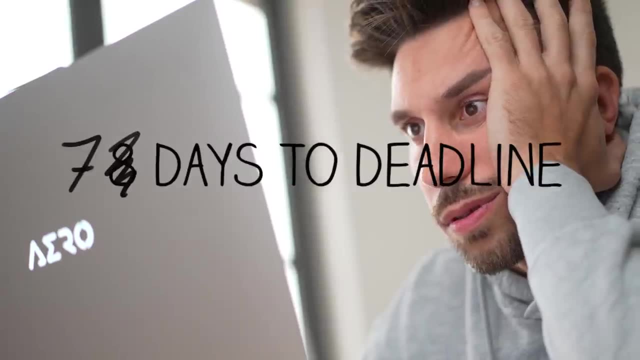 Can a person with no animation experience- that is, me- actually create an animation movie? I'm not sure, but I just signed up for a contest online and I have 8 days to make one. Eh, actually 7,, because I spent the first day trying to at least understand how everything works, unsuccessfully. 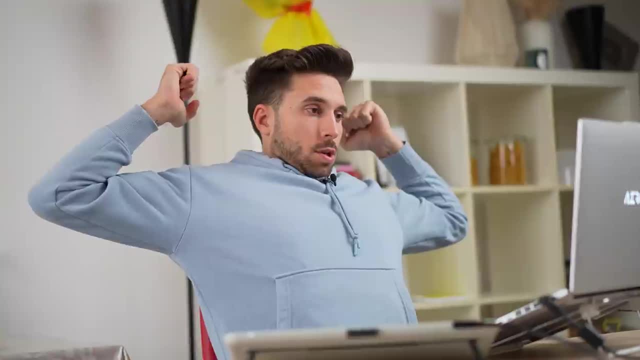 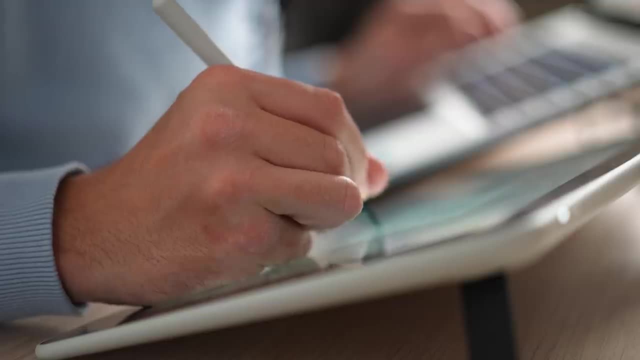 7am, day 2.. I woke up, brushed my teeth, had breakfast and I was excited to start. Alright, let's do this. The second day I actually decided to start practicing drawing the first lines. Sounds obvious, but the first step of animation is drawing. 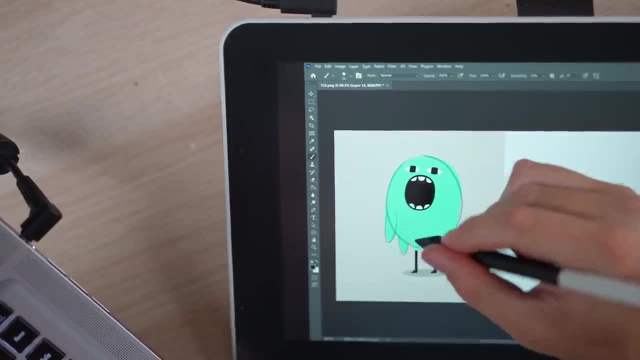 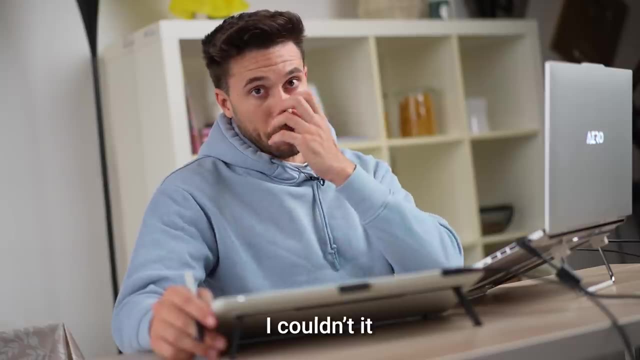 I learned this a while ago: If you want to draw anything, you need to break down the subject into simple shapes And after that you can start worrying about the details. And I thought I found a simple subject, but I couldn't do it. I hate circles. They are so freaking hard. 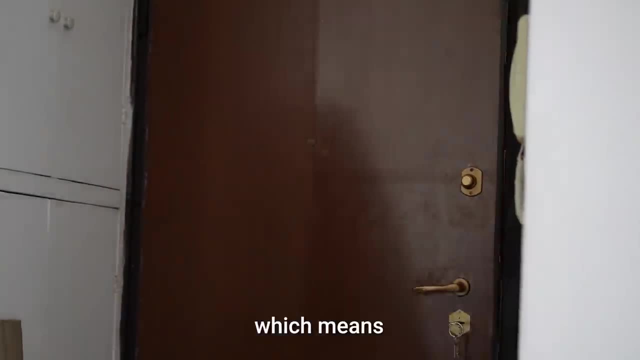 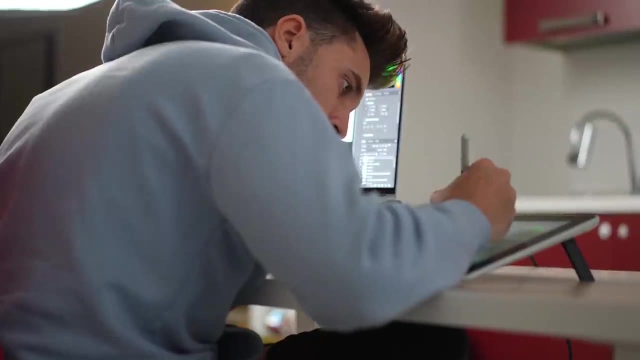 I needed to find an easier subject. My girlfriend left this morning, which means it's just me, my laptop and my beautiful little, sweet cat. I think I'm gonna draw you, And I actually decided to practice for a while using my cat. 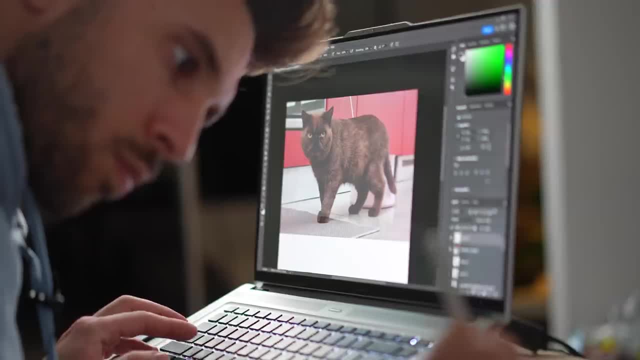 First step, taking a picture of Cookie- His name is Cookie- Then I broke down his body into shapes, Not literally- And then I added details And it turned out good. But it took me hours to get to this point. 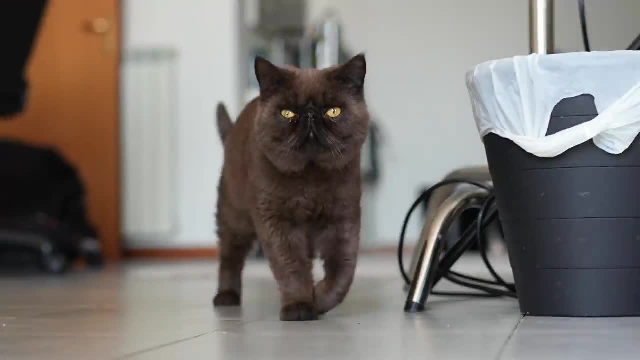 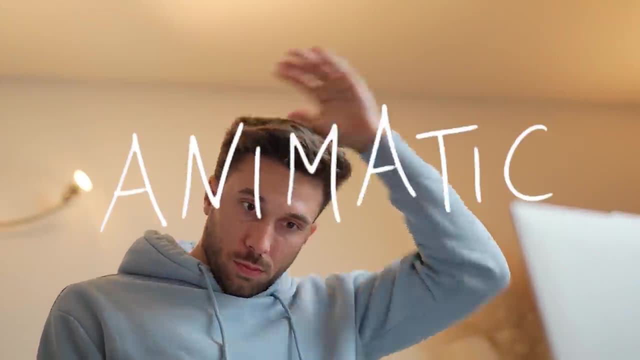 Now to animate Cookie, I should draw him again 24 times in slightly different positions, all to create a single second of animated movie. And that is the moment I realized I would never make it that way. I had to use animatic, which always consists in a series of images played in a sequence. 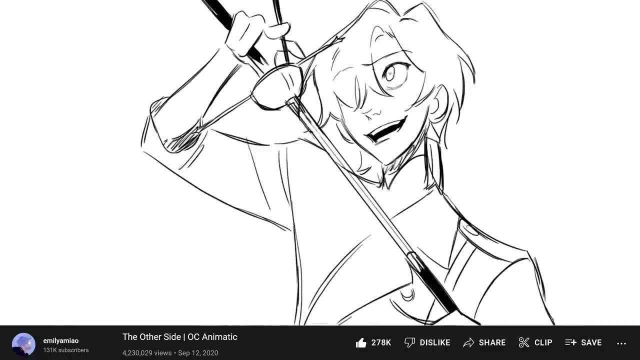 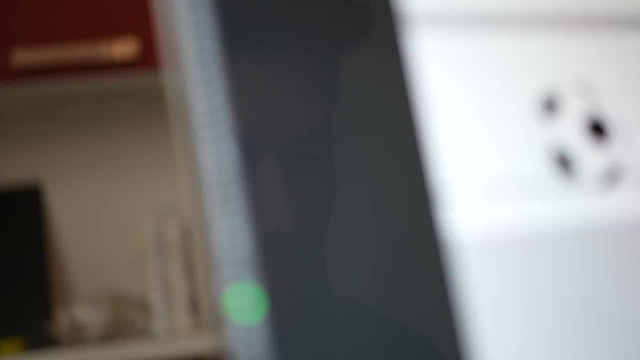 But instead of drawing 24 frames each second, each frame will last a few seconds. It's beautiful, it's way faster and it's literally the only way I can finish my movie in time. I practiced a bit more and after two hours my masterpiece was completed. 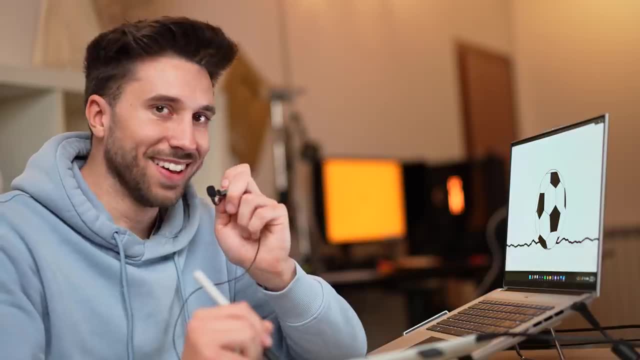 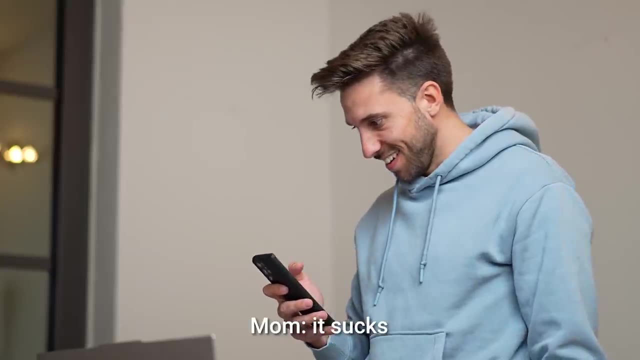 I spent two hours for a four seconds animation. It looks great, It's beautiful. My mother called me again asking me what I was doing. I told her I drew a ball. Anyways, I kept working or leaving until I couldn't work anymore. 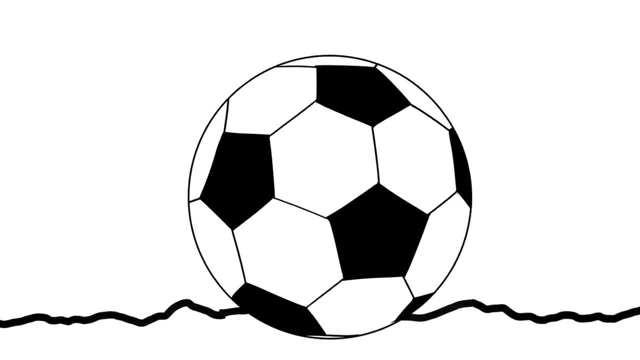 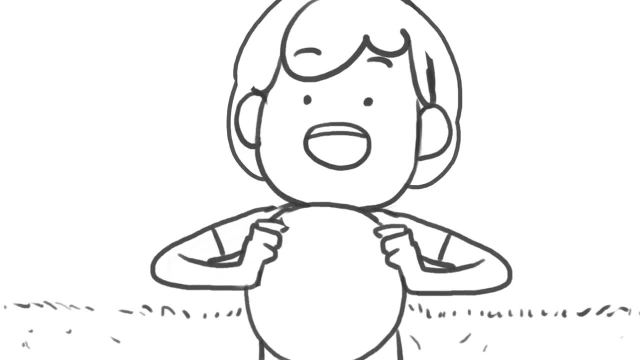 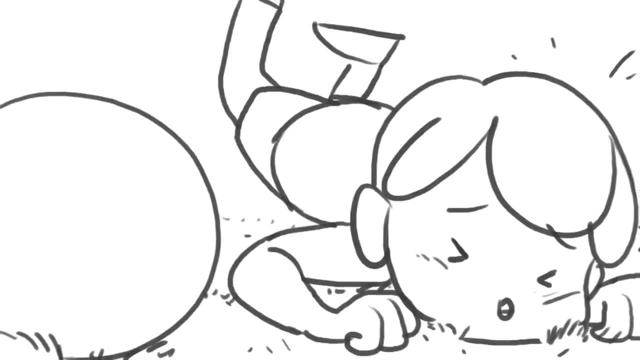 And then I fell asleep on my table. A ball- Hey, look at him, He has a ball. Hey, kid, come here, Let's play. Sure, I told you not to let him play. Come on, kid, go away. You're so bad. 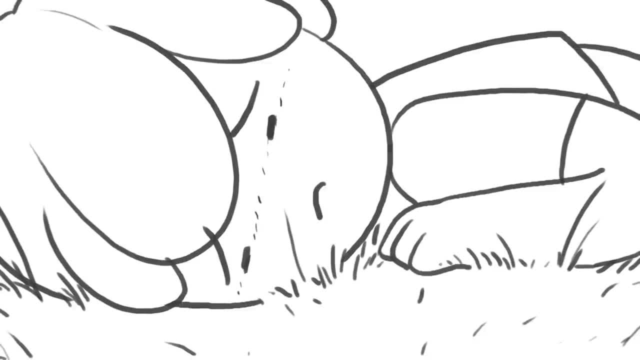 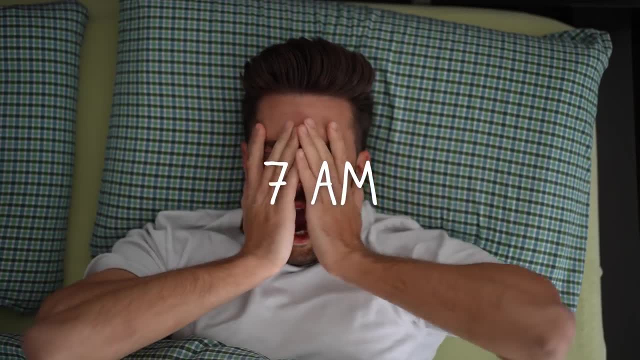 Move And we'll keep the ball. I woke up at 3 am and when I realized what it was and what time it was, I decided to go to bed. 7 am, six days left. I woke up running, washed my face and I ate this. 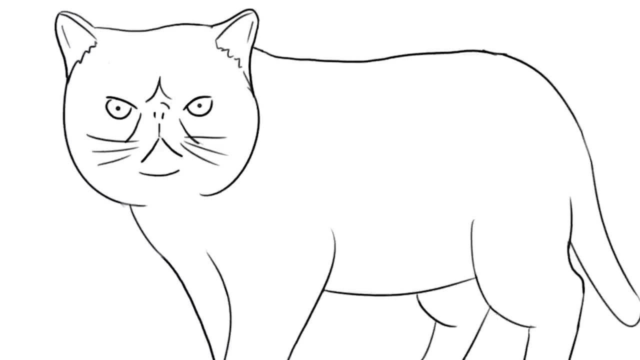 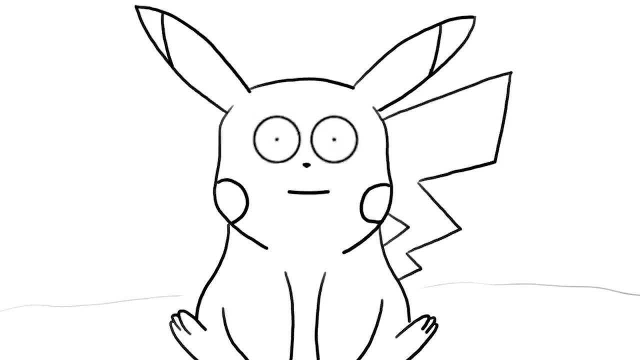 The next thing I want to learn is giving more emotions to my characters, And that's what I'm going to do, And I probably can achieve that by drawing actual eyes instead of dots. So then I tried a few styles. Some were too simple, some were way too complicated, but you can always find the perfect one for your characters. 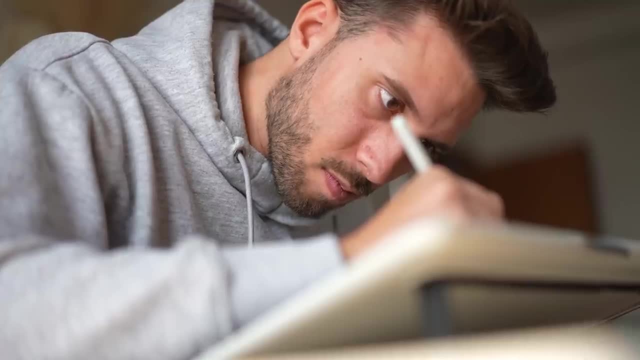 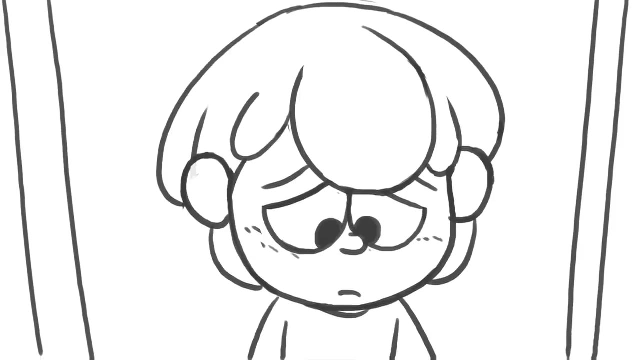 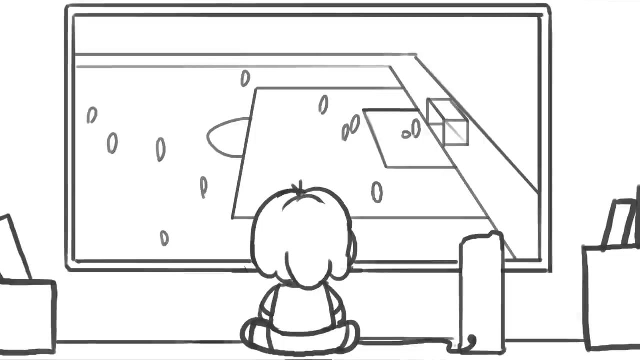 I kept working on the movie for three hours straight, as if my pants were glued to the chair, And, honestly, I was starting to feel the pressure. I will never step in a football field ever again, Mom, Anyone. Yes, I love this game. 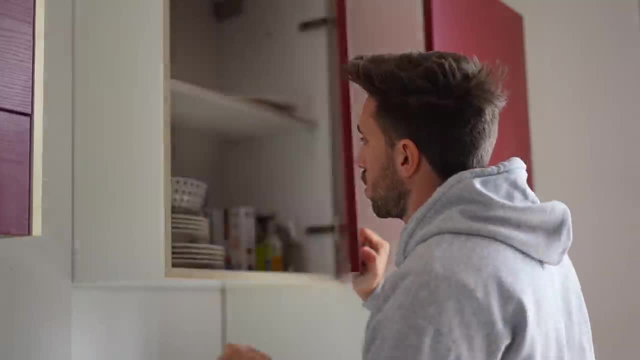 You know, I promised myself I wasn't going to order junk food this year And I've been actually keeping a healthy lifestyle by working out and cooking everything by myself. But I really didn't have time. today It's already 3 pm. 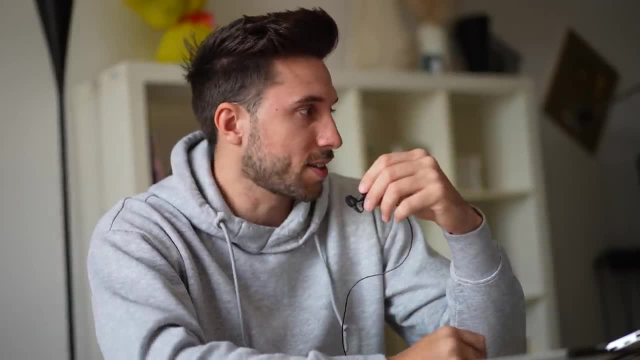 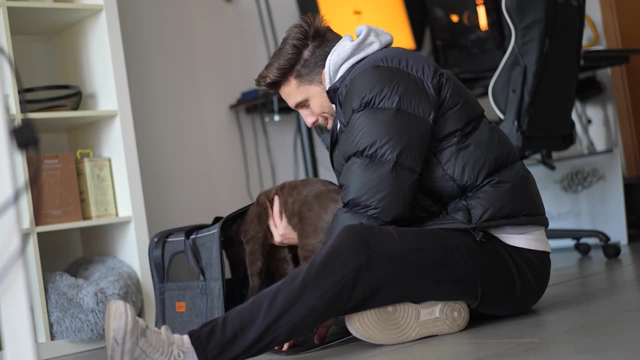 And if I want to finish the contest on time, I need to be so much faster than this. And then I got a call from the vet. He reminded me that I had an appointment for Cookie that I completely forgot about. I left home. 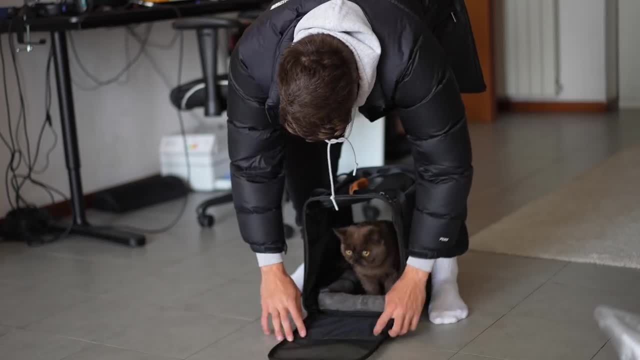 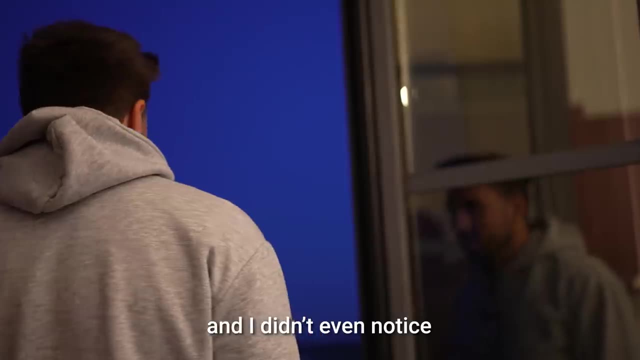 Cookie wasn't happy. Vet Cookie was even less happy Home. My two days animation experience taught me something already: Animation has the power to make time fly. It's already dark outside and I hear even noise. Anyways, I worked all evening. 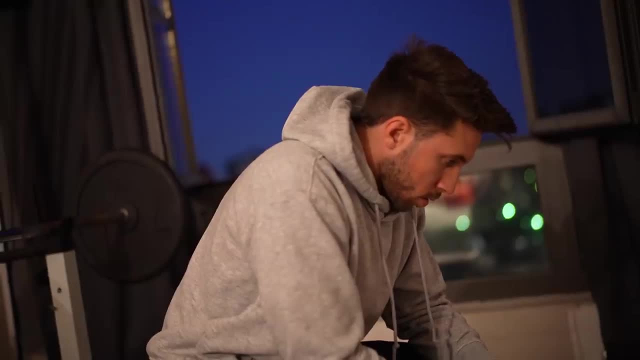 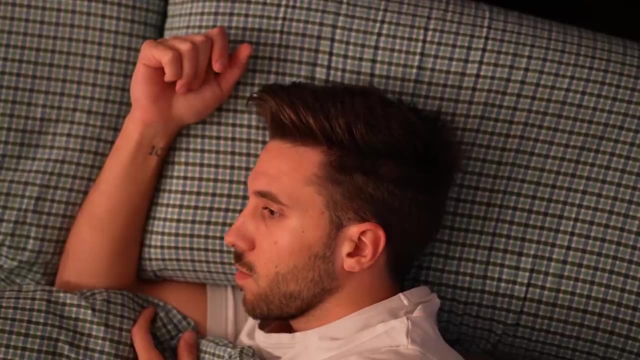 And I watched an animation tutorial while working out, Which means I worked out really bad. I kept working and then at midnight I stopped. I promised myself to go to bed no later than 12 pm this year And I need to maintain that habit. 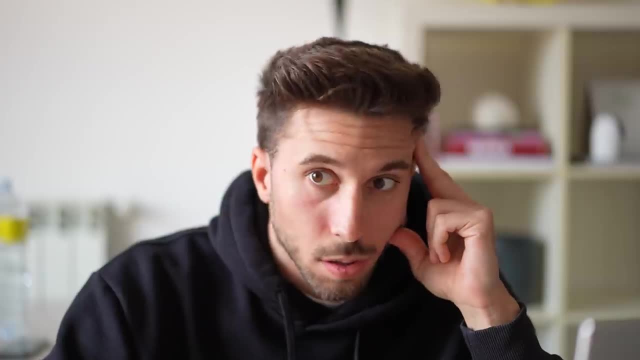 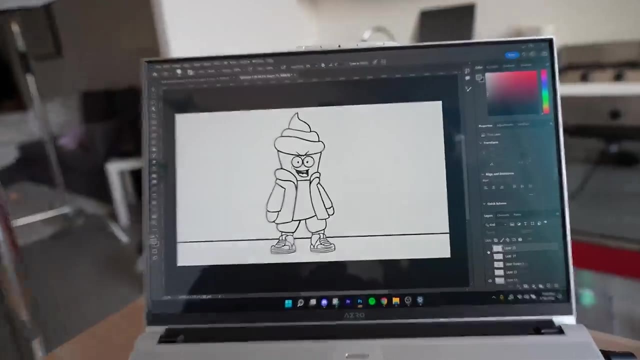 7 am, Five days left. I washed my face. I'm not even sure if I had breakfast. My drawings look like if a four-year-old kid tried to sharp a pencil against a sheet. I just came up with that. I'm joking. 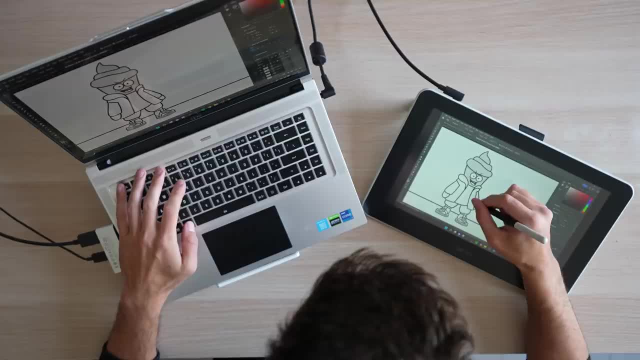 It's pretty cool, But I need a bit of realism, And so I decided to add a grayscale to my drawings, Starting from this Ice cream, I guess- And I even added shadows. at the end. I was pretty proud of it. 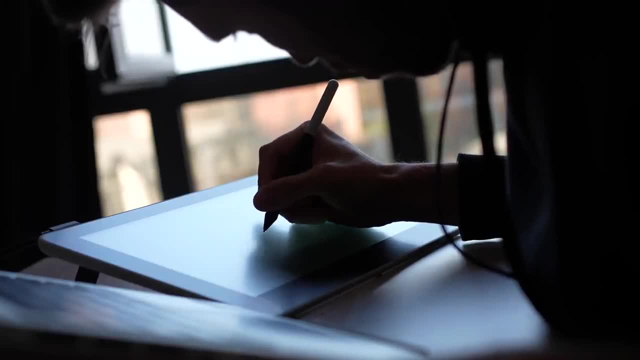 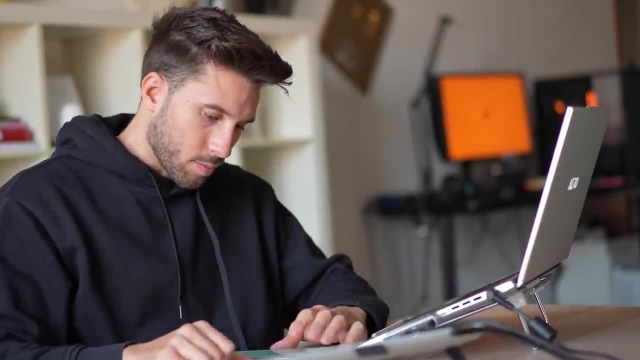 Then I started working on my movie once again Because I knew I was terribly late. Five days is nothing to create what I had in mind. After a while my mom called me, But I felt like I didn't have time And I was probably right. 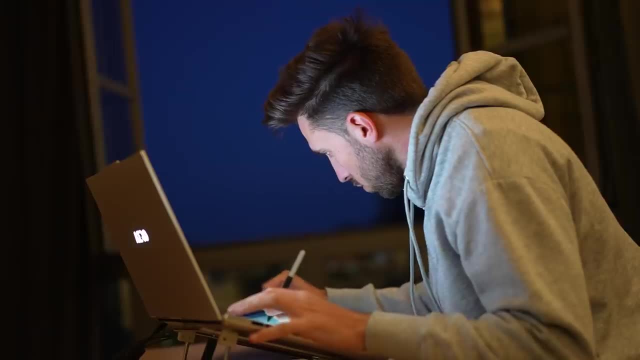 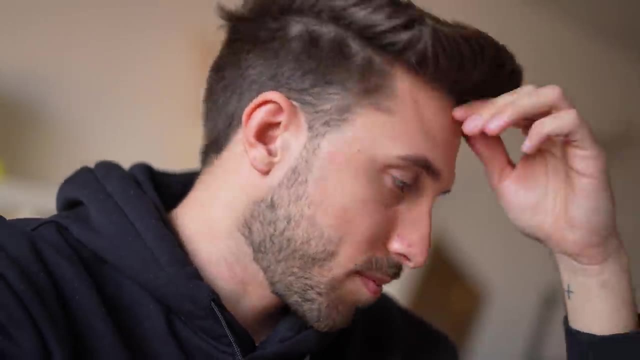 She doesn't get it. I feel like nobody gets it when I'm in these situations And I need to work hard And I already worked, And I always end up feeling dumb. I think I'm the only one who realizes that I didn't work out. 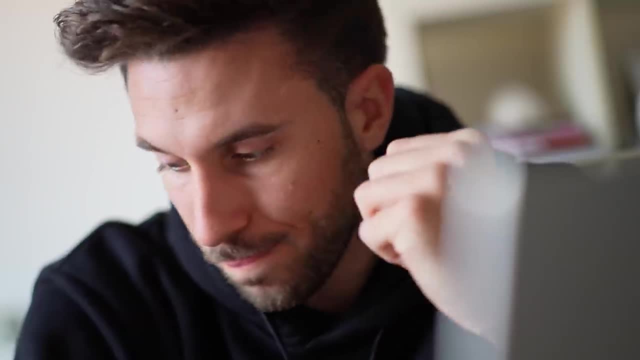 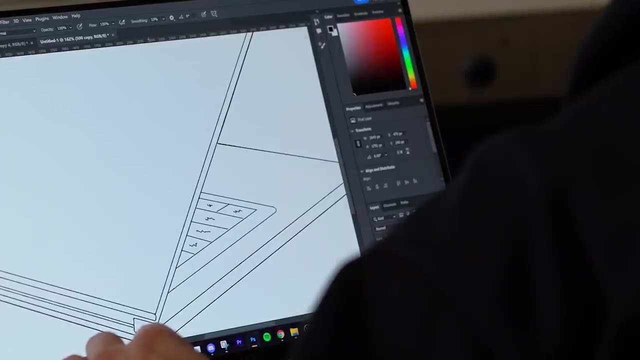 I didn't eat well And, honestly, nothing mattered. I just wanted to work on the movie, But I really felt bad for this guy. Gigabyte sent me this laptop, which is absolutely great, And in return I promised I would deliver a great animation work. 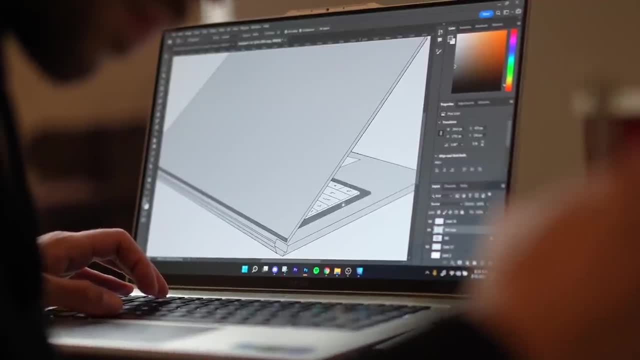 The problem is, I didn't even know if I could do it And so, to pay respect, I tried to draw it. I know basically nothing about PCs, but this is insane. That is the most beautiful display I've ever seen on a laptop. 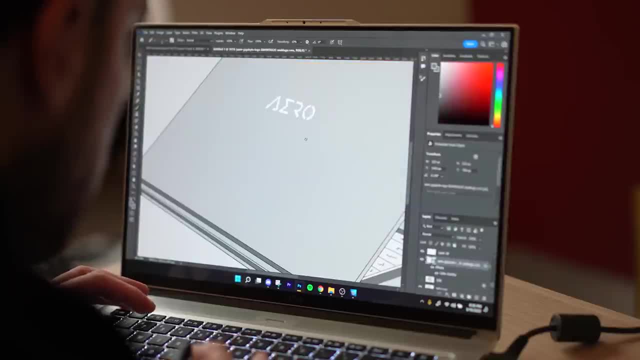 Insane GPU And it's equipped with a 12th gen Intel processor. So, basically, if you're a content creator and you're looking for a really cool laptop, this one is for you. Then, at 3 AM, I realized it was 3 AM. 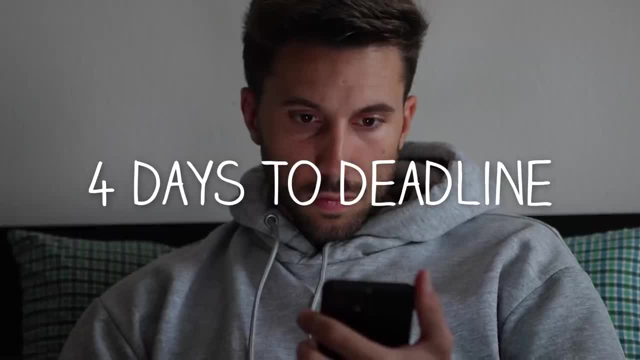 And so I went to bed 11 AM, four days left. I was feeling down, But music fixes problems. I drew all day and I felt great, I was making progress And I was also kind of starting to like my drawings. 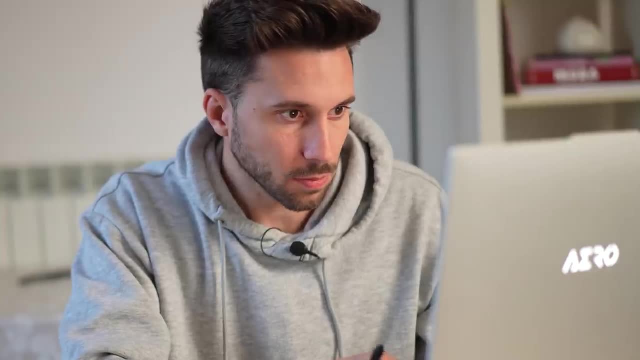 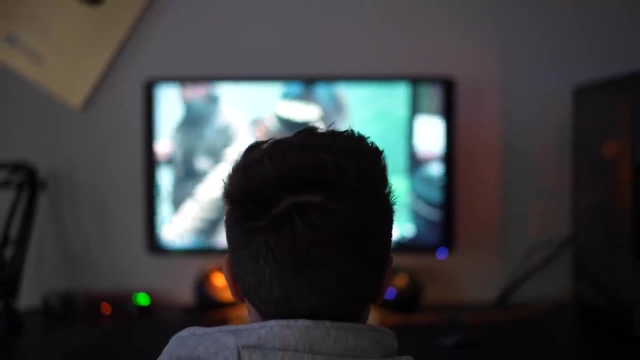 And the next morning my girlfriend was going to come back, which is great Because I was starting to feel lonely, I guess, And at 10 PM I even found the time to watch a movie. Then I realized I literally missed dinner. 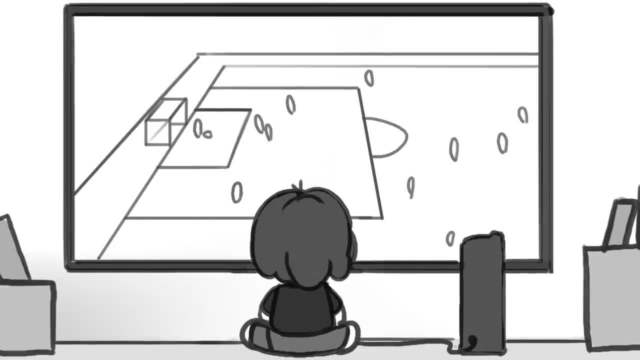 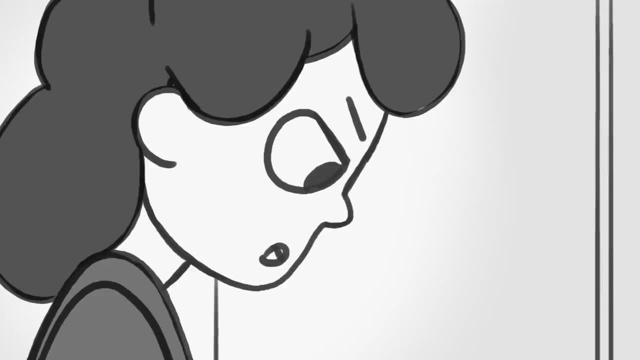 Come on, I'm getting out of this place, Mom. you've been playing all day. You need to stop. Come on, Mom. Only one more. No, you need to stop now. It's a beautiful day. go out. 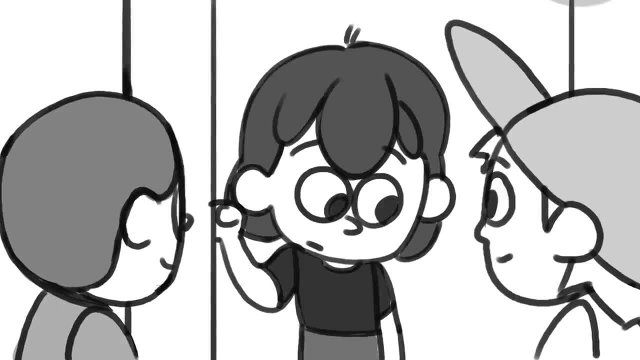 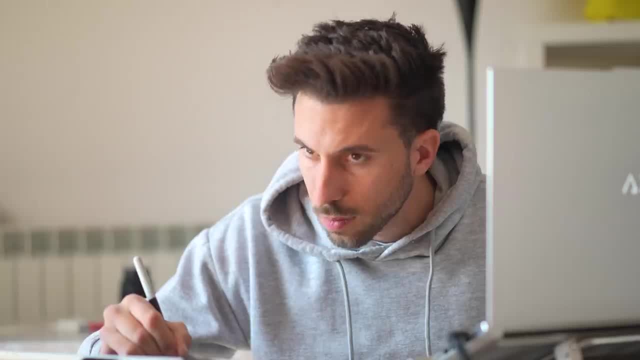 Hey, Come play with us. I'm not sure, guys. I don't feel really well. Come on, we're going to wait for you there. Three days left till the deadline. I ate maybe. I immediately started doing a bunch of stuff, and that's exactly what I'm talking about. 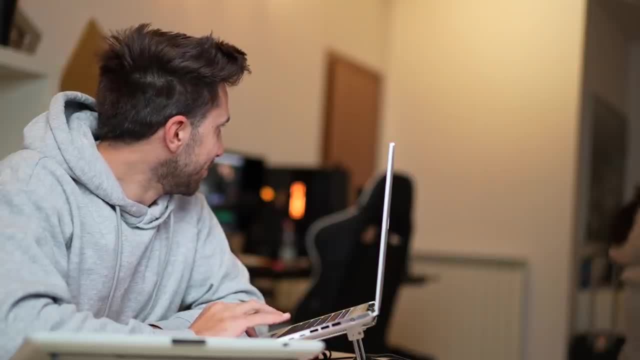 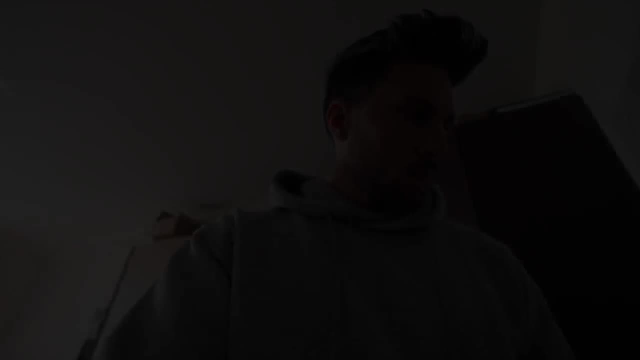 Yes, I know Exactly what I had to do. when my girlfriend arrived, I was genuinely full of happiness, but time, that's what I didn't have. Then I decided to go anyways, and we ended up fighting because I mean, I was there But I wasn't really there, and she told me I was obsessed. You know what I did? 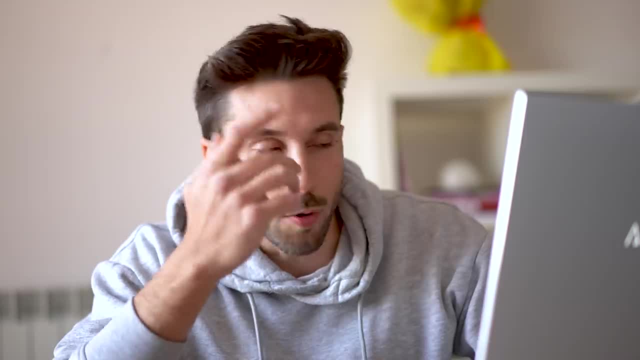 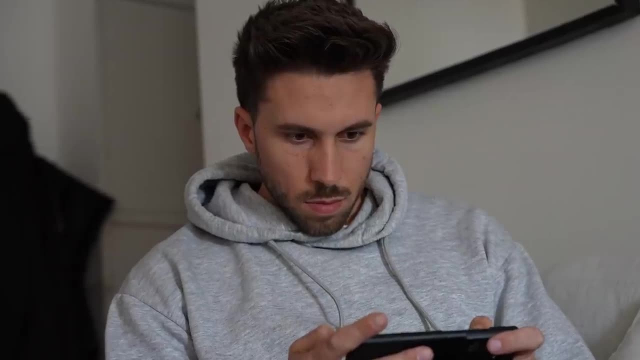 I went back to my PC, basically proving she was right. You know what? I Didn't want to do anything. I stopped caring about the contest, about animation, about anything in general. I just wanted to play a football game on my phone. I used to love doing this when I was a kid and now I felt like I jumped back there playing a game. 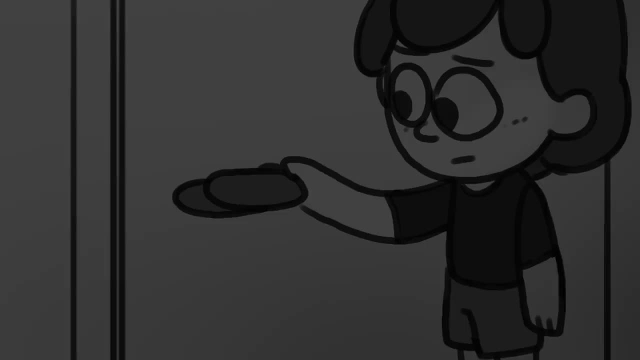 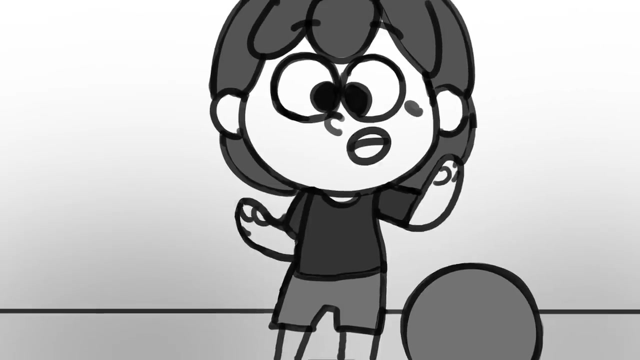 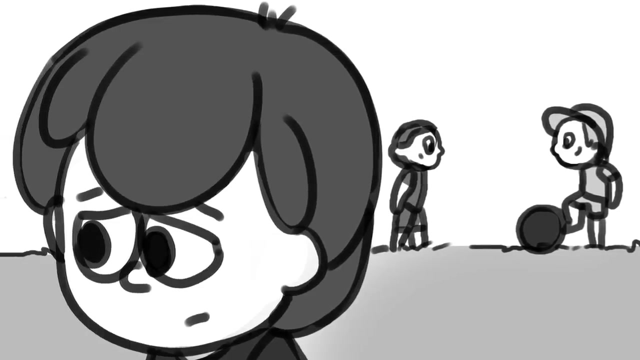 alone after 17 years. Maybe that would be actually fun. I think I'm gonna go. Hey guys, I'm here. Can I play? I'm sorry, We already got the whole team All right. No worries, guys, Maybe I don't need anyone else. I can play by myself. 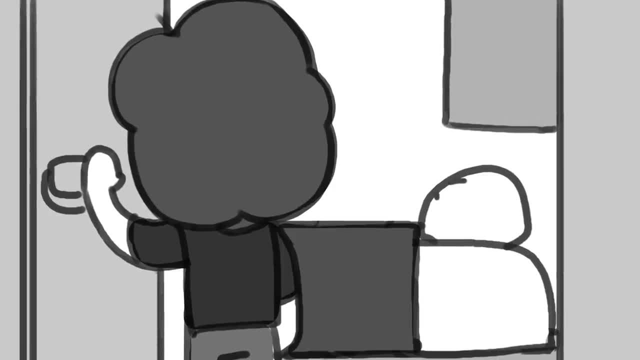 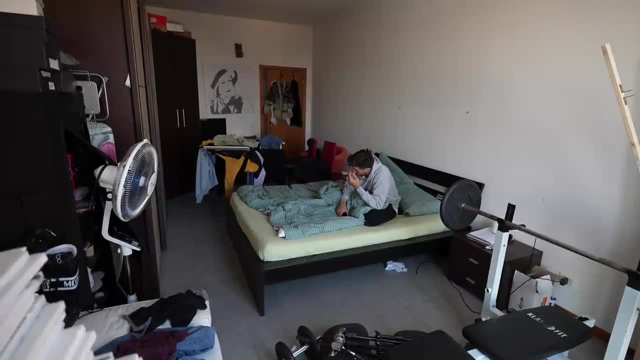 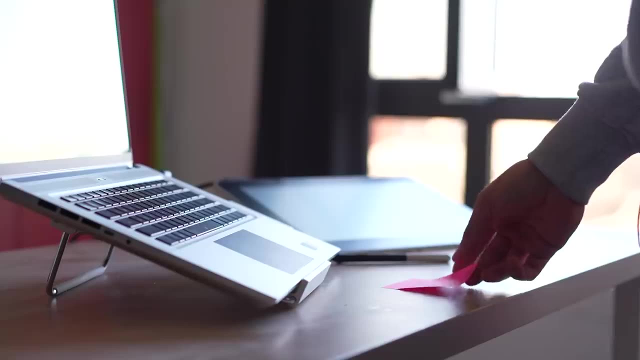 Oh, Two days left. I woke up late and the house was empty, kind of. I felt really bad. I didn't take a shower in three days and This is gonna be the fourth. and then I saw this. I understand how you feel. I don't want to fight, sent her a message, and then I also called my mother to let her know that I was still alive. 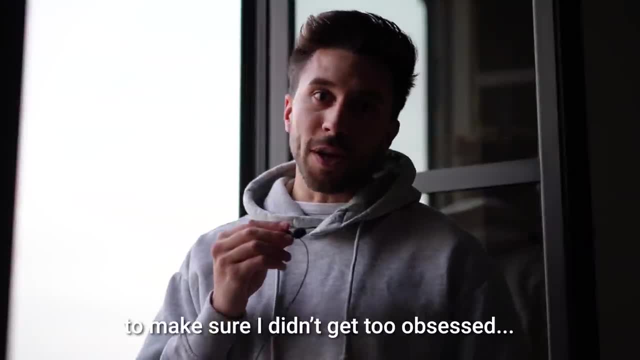 Maybe it's not that the others don't get how I feel. Maybe they were just trying to make sure I didn't get too upset. Maybe they were just trying to make sure I didn't get too upset. Maybe they were just trying to make sure I didn't get too upset. 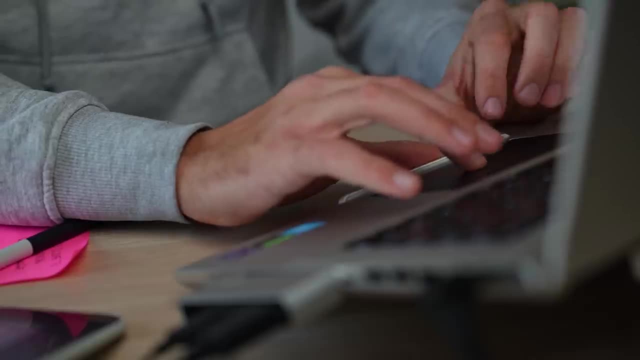 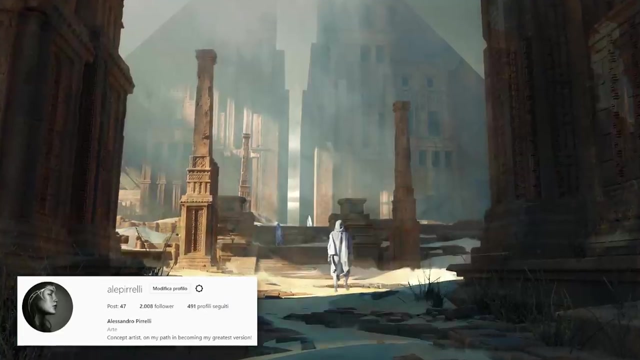 Which I did, and so, with two days left, I give up on the contest, But I'm still finishing the movie and I'm gonna show you the final result. I'm not giving up on that. a friend of mine, who's an actual monster- a drawing- is gonna help me out doing it. 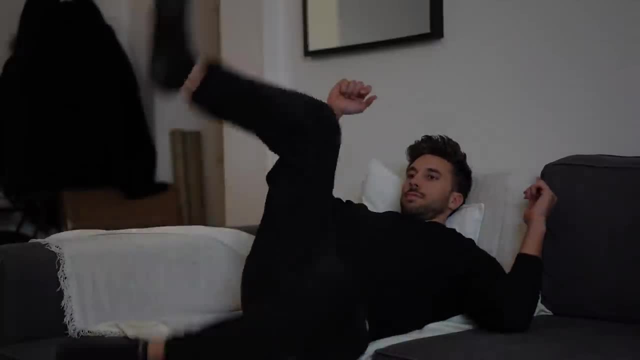 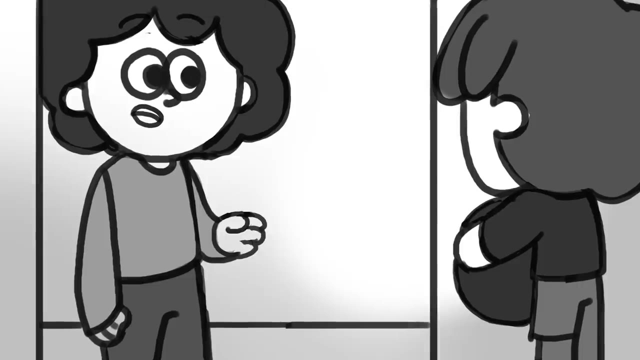 And just like that, I finally had time to do Absolutely nothing. Hey kid, here's your ball. I'm sorry for my friends, Sometimes they're Asymmetrical. you keep practicing and you'll be great one day. actually. come with me, Let's go play. 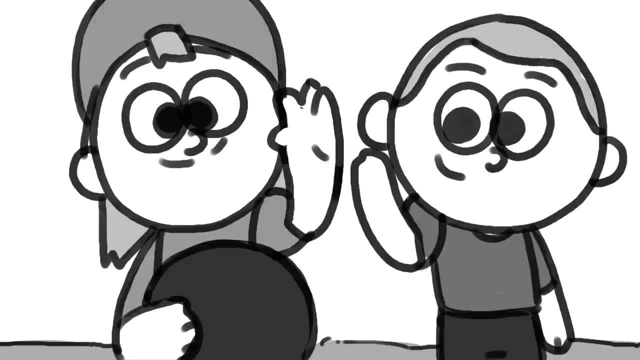 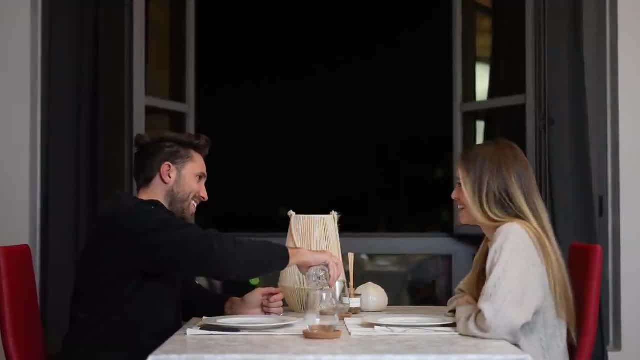 I'm sorry for the last time today. We are going to play all day. It's good to see you. We're sorry for the last time today. We are going to play all day. In this moment I realized something. I was happy, but not only because it was with my girlfriend. 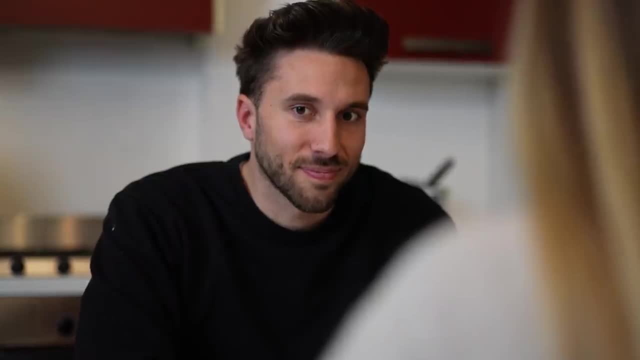 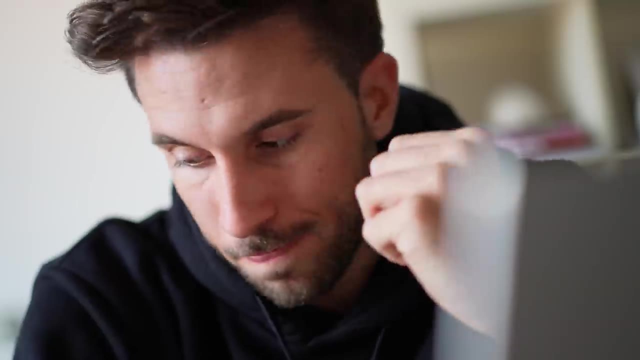 This experience taught me something way bigger than animation, and only now I actually get it. There is a person that is always there for you And I mean we should respect this person, But we just tend to forget that. this crazy thought that I had while washing my hands is that all our lives, even if we 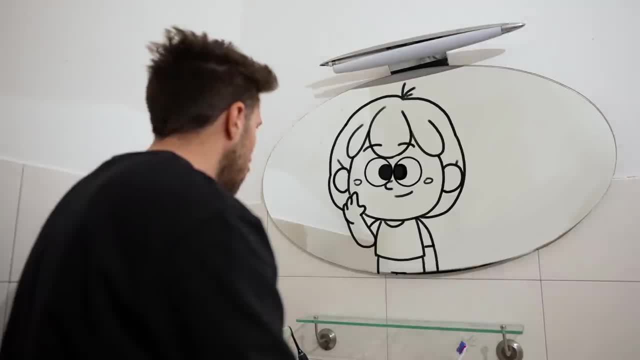 Are alone Sometimes. we are actually never really lonely. Mike, let's go.